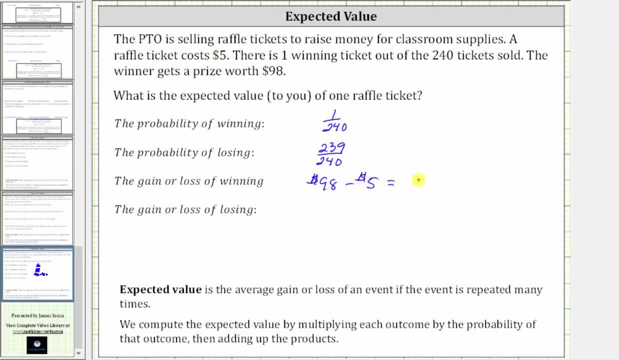 minus the cost of the ticket, which is $5, and therefore the gain is really $93.. And then the loss of losing would be the loss of the price of the ticket, which is $5.. To indicate the loss, we use negative $5. 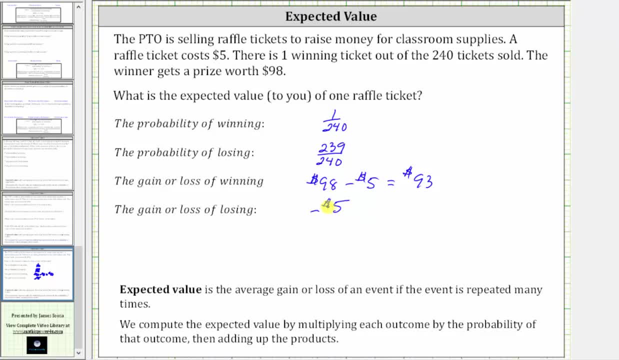 And now we have the information we need in order to determine the expected value. Again, the expected value is equal to the sum of the products, of the outcomes and the corresponding probabilities. Let's consider the first outcome of winning Again. if you win, you gain $93, so we have $93,. 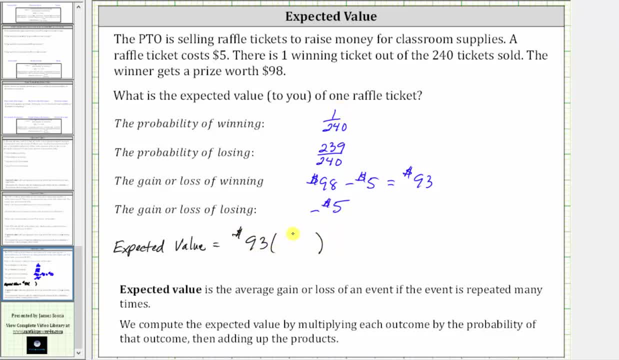 and we multiply by the probability of winning, which is one divided by 240, and then plus the second outcome, which is $93.00.. The second outcome is that you lose. If you lose, you lose $5, so the outcome is negative $5. 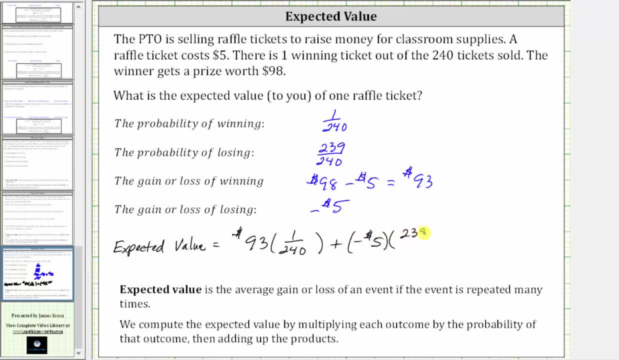 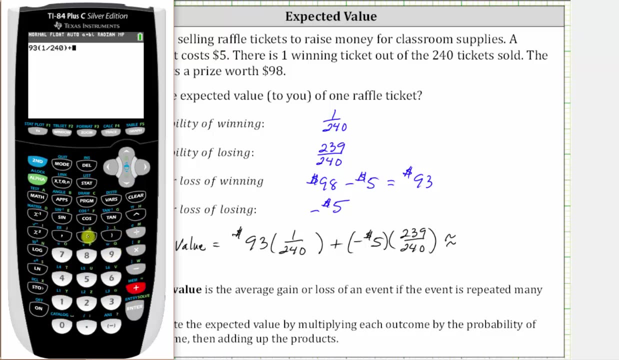 times the probability of losing, which is 239 divided by 240.. And now we determine the sum of the products using the calculator and round to the nearest descent. So we have 93 times one divided by 240, plus negative five times 239 divided by 240. 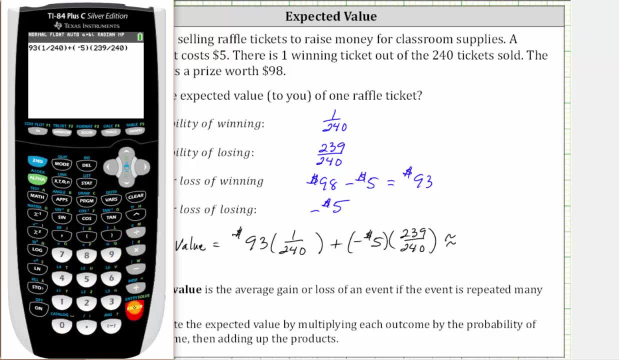 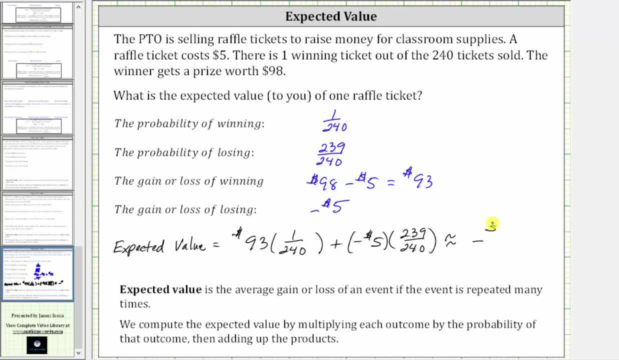 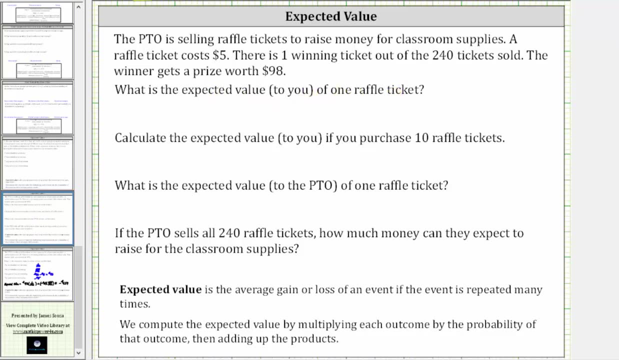 And enter To nearest ascent, we have negative $4.59.. So, going back to the first slide, the expected value to you of one raffle ticket is negative $4.59, which means you can expect to lose $4.59 for buying one raffle ticket. 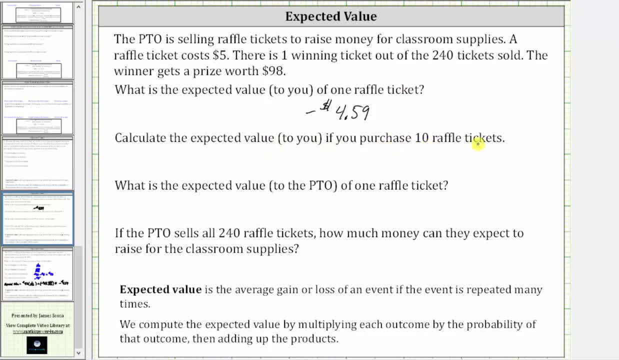 Next we're asked to calculate the expected value to you if you purchased 10 raffle tickets. To calculate this, we multiply the expected value of negative $4.59 by 10.. So negative $4.59 times 10 is equal to negative $45.90.. 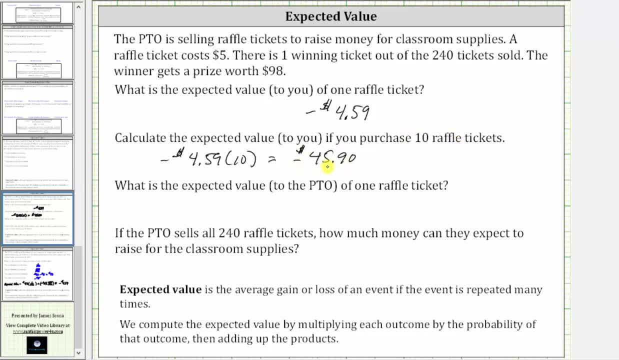 So if you buy 10 tickets, you can expect to lose $45.90.. So if you buy 10 tickets, you can expect to lose $45.90.. So if you buy 10 tickets, you can expect to lose $45.90..